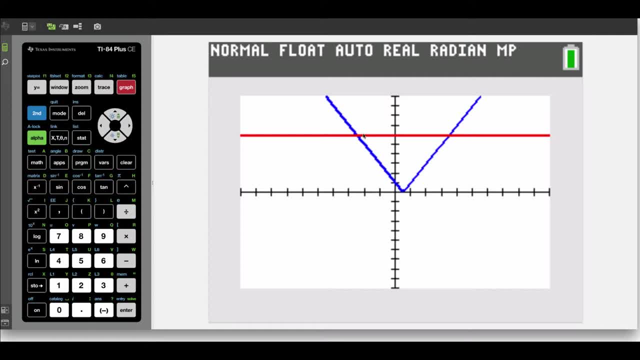 looking for the intersection. So we're looking for where our graphs cross each other and there are two places where these graphs intersect. So we're going to look at the intersection and we're going to look at where those trac-trace купics meet. We've got that blue absolute value of a. 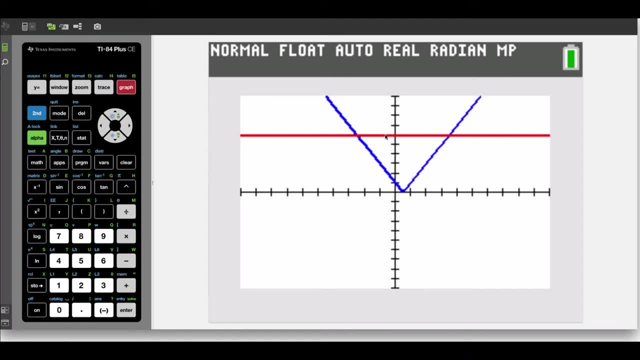 v-shaped graph and our horizontal line is 6.. So we've got an intersection on the left hand side and the right hand side. To find those intersections we're going to use our calculate option. So we're going to go lost trace. and now option number 5 is intersect. 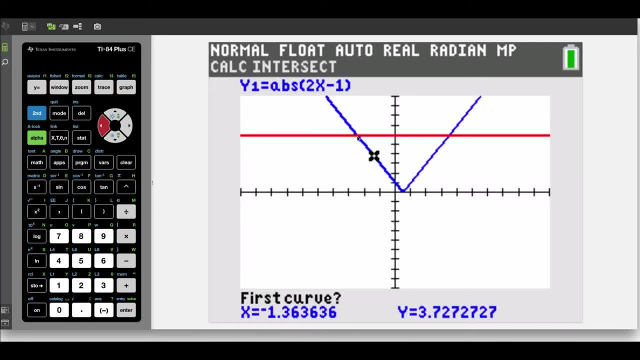 So we're looking at our graphs. There are two intersection points, So I'm going to start with this one on the left hand side, So I'm going to arrow left over to it. Now it asks for our first curve, So we want to make sure that that's là anders. 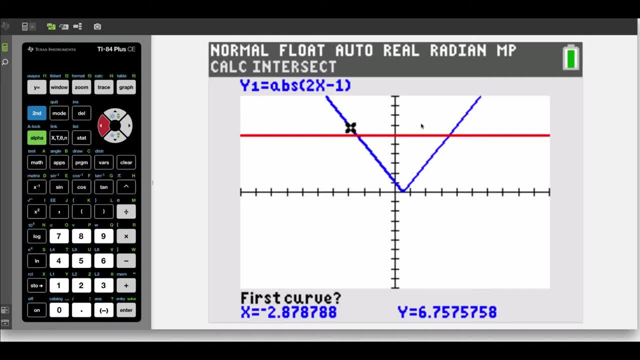 for our first curve. so we want to make sure that we're on our absolute value graph, our blue graph. I hit enter. then it asks us for our second curve. so I make sure that it's switched over to my red graph. hit enter. we can take a guess, but we don't have to. we can just hit enter one more time. so. 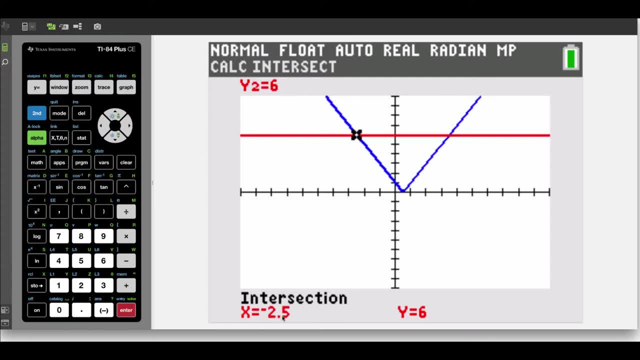 the first intersection point is at: x equals negative 2.5, y equals 6, meaning that the x value there is negative two and a half. so that's one of the solutions. now if we want to find that other solution, we're going to have to hit second calc and then intersect one more time. so option number: 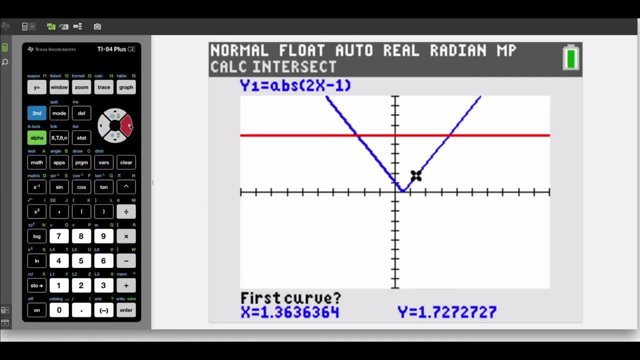 five. now to get the other intersection point, I'm going to have to move my cursor over closer to that point, first curve, just like we did before. make sure that I'm on my absolute value graph. so I'm going to arrow over just a little bit to show that we are on that v-shaped graph. 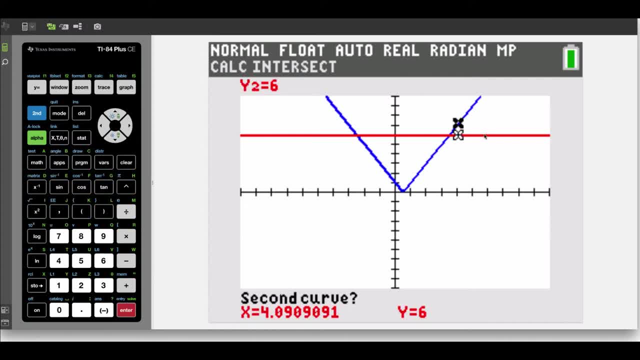 hit enter, then make sure it switches to the other curve that we're looking at, so that horizontal line hit enter again. we can take a guess, but we don't need to. we can just hit enter one more time. so there's another intersection point: at x equals 3.5, y equals 6, so at three and a half we also have a solution. so, going back to our 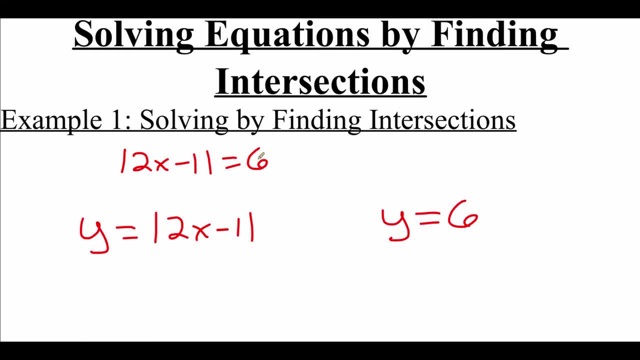 equation where we've got the absolute value of 2x minus 1, equals 6. there was two answers. one of them was at x, equals negative two and a half, and the other one was at x, equals three and a half. so those two x values are the solutions to this.